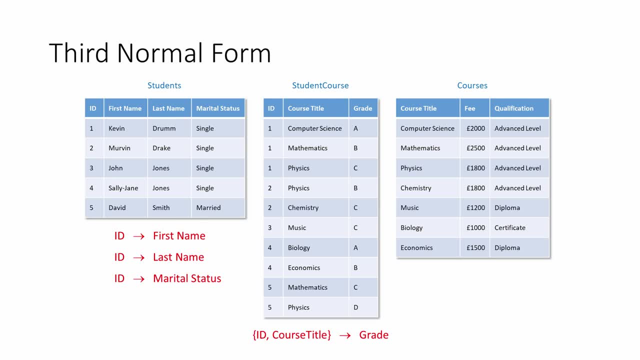 It's OK to have functional dependencies in a table in order for it to be in third, normal form. In fact, it's absolutely necessary. Every non-key attribute of a table must be fully functionally dependent on the primary key. If it was partially dependent, the table 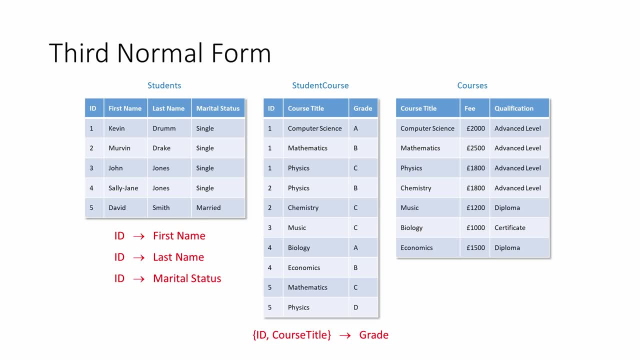 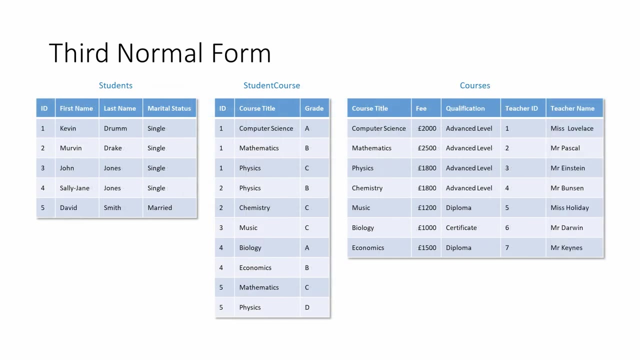 wouldn't even be here. So what's a transient functional dependency? These are not allowed in third normal form. Let's add some more data to the courses table to help make this clear. The course title is still the primary key of the courses table. It's unique for each. 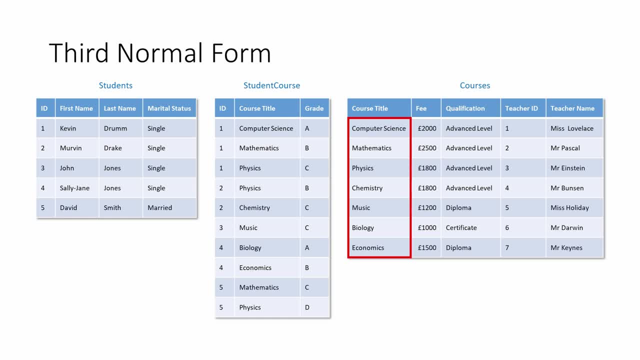 course. It certainly belongs here. As an aside, if there were two courses with the same course title, perhaps a Computer Science A level and a Computer Science B level, Then you'd have to rethink the primary key, perhaps by giving each course a unique. 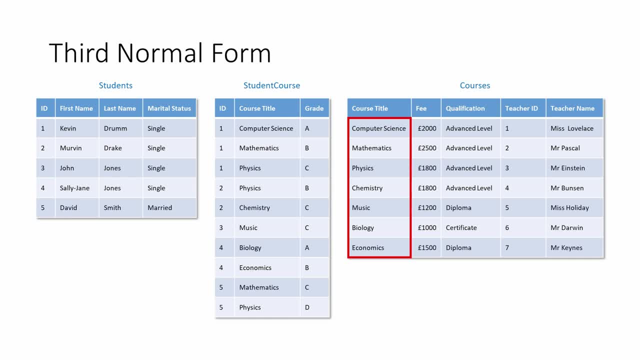 code, But let's proceed on the basis that each course title will always be unique. The fee and the qualification are both attributes of the course title. They're functionally dependent on the primary key, so they belong here. But the teacher ID and the teacher name columns seem a little out of place. Each course is 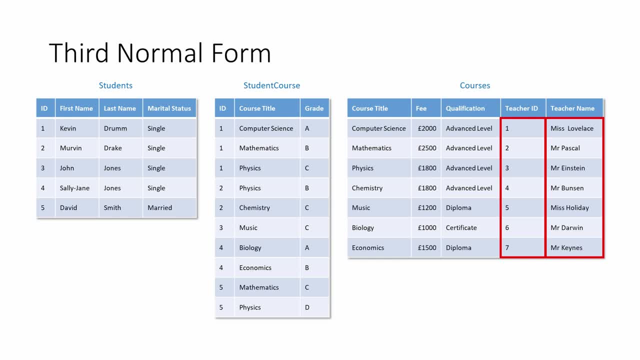 always taught by the same teacher According to the teacher ID and the teacher name columns. each course is taught by the same teacher According to the teacher ID and the teacher the same teacher according to this data at least. so you'd be forgiven for allowing. 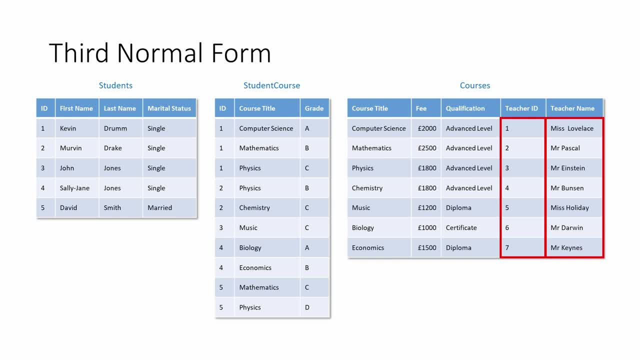 them into this table. in the first place, Teacher ID is an attribute of a course, and it's functionally dependent on the primary key. Teacher name is also an attribute of a course, and it too depends on the primary key. There are no partial dependencies on the primary key here, so the table is indeed in second. 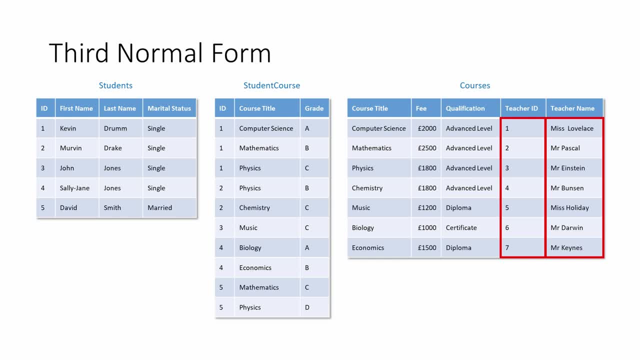 normal form, But there's a potential problem. If you decide to change the teacher for a course, then you have to change both the teacher ID and the teacher name. They are functionally dependent on each other. This is not ideal because, as you know, editing mistakes can lead to inconsistencies in the 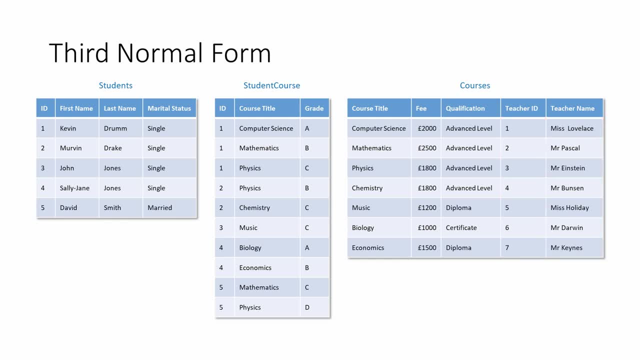 data. If you change one of the course titles, it becomes a different course. So again you need to change the teacher ID and the teacher name. To put this in technical jargon, The teacher ID is functionally dependent on the course title and the teacher name is. 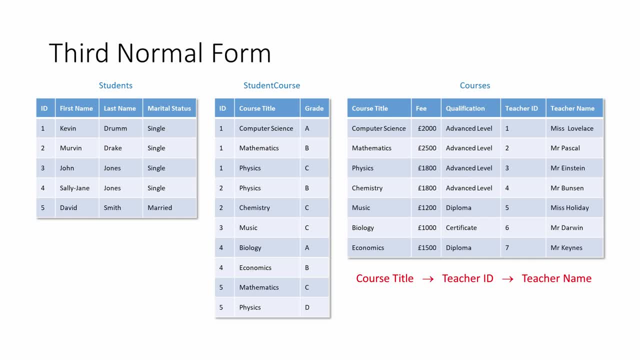 functionally dependent on the teacher ID. So there's a transitive dependency between the teacher name and the course title. Something depends on something which depends on something else. It's also true to say that the teacher name is functionally dependent on the course title. 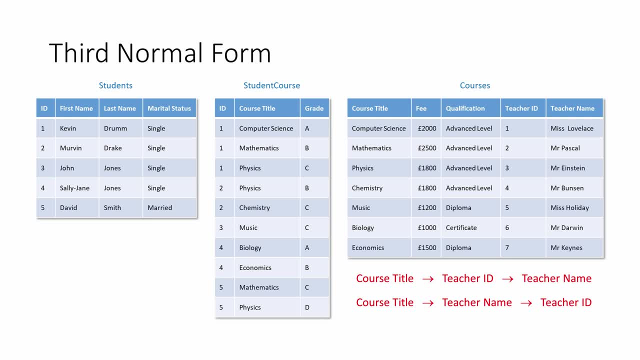 and that the teacher ID is functionally dependent on the teacher name. so there's a transitive dependency between the teacher ID and the course title. teacher ID and the course title. it's just another way of looking at these particular data. whichever way you look at them, there are transitive functional. 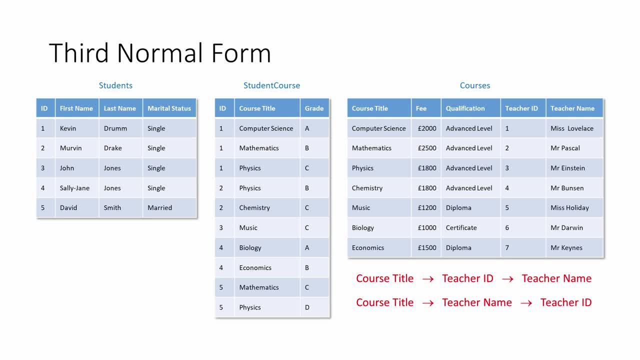 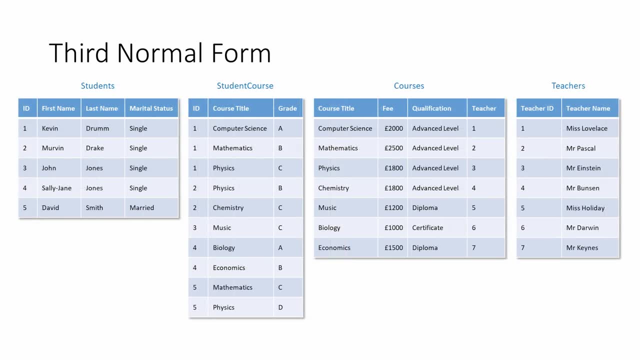 dependencies here, so the courses table violates third normal form. this is how to solve the problem. you need a separate teachers table. the teacher column in the courses table establishes the relationship with this new table. none of these tables contain transitive functional dependencies. the database is definitely in third normal form. 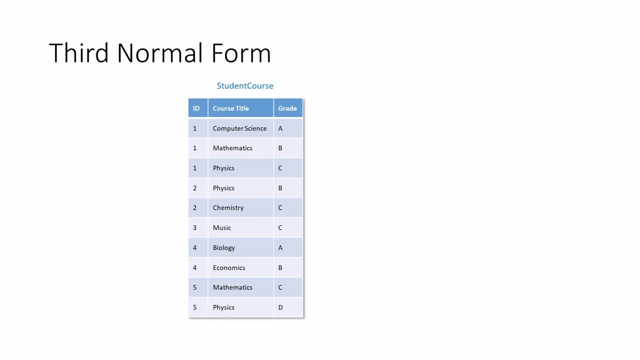 another example of a transitive functional dependency would be if the student course table contained an exam mark as well as the grade. the grade is derived from the mark. now, arguably, you shouldn't store any attribute in the database if you can calculate it from something else. nevertheless, 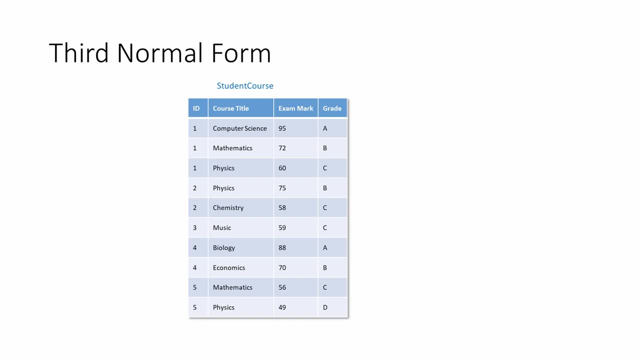 let's suppose you had good reason to store both the exam mark and the grade in this table. if you change the value of the primary key for one of these records, it's a different student course combination, so you need to change the exam mark and the grade to match. the mark is functionally dependent on the 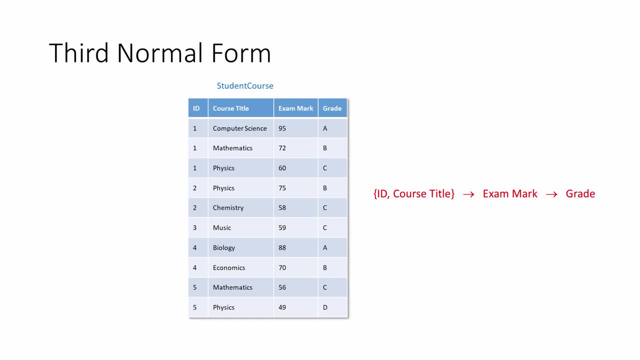 primary key and the grade is functionally dependent on the mark. there's a transitive functional dependency between the grade and the primary key. strictly speaking, in order for this version of the table to be in third, normal form, the mark and the grade belong in a table of their own, perhaps a. 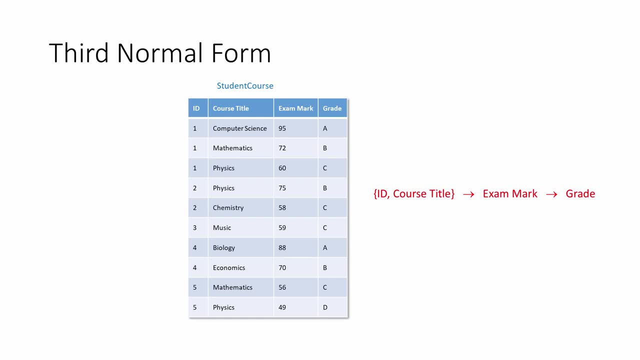 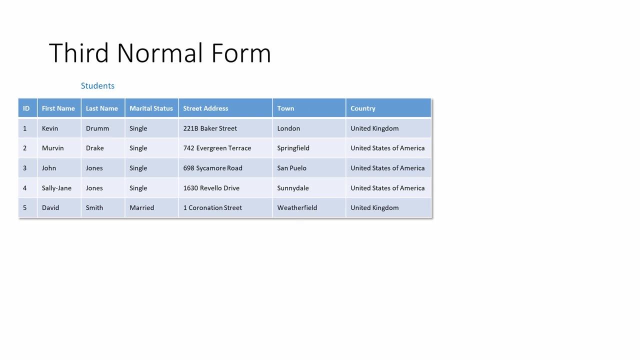 table called results. let's stick with just the grade in this database. now take a look at this version of the students table. a purist might tell you that if you were storing postal addresses in the students table, then these should be moved into another table, every part of the address.